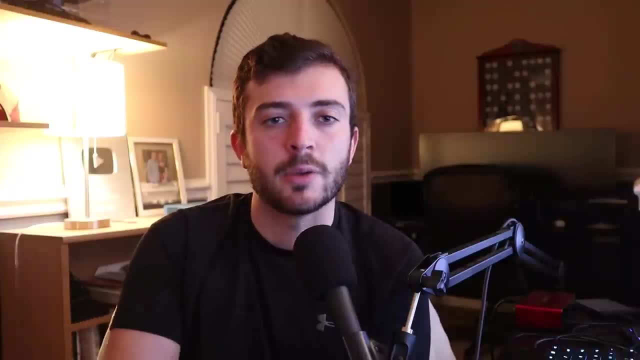 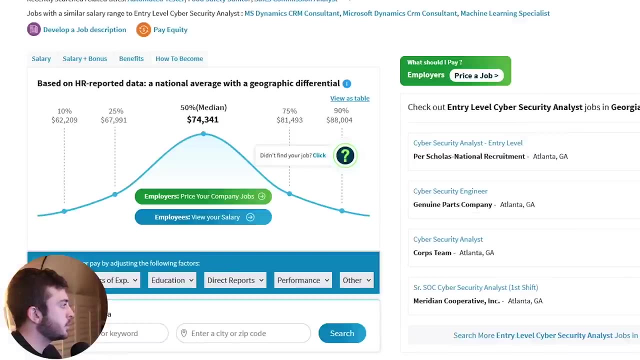 wrong on that point, But it still doesn't think about entry-level cybersecurity jobs. Looking at or Googling entry-level cybersecurity jobs, what you're going to find is a median that doesn't necessarily an average or mean, but a median salary of $74,000, which is pretty good for starting out. So ultimately, the likelihood of an entry-level job in cybersecurity being above six figures is going to depend on multiple factors: the type of company, qualifications, certifications, previous experience, the way or where you are living, and much more. I'm stating pretty much the obvious here. I'm saying this as a cautionary, so have the right. 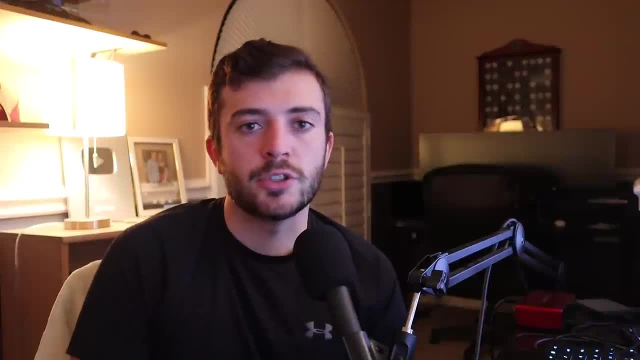 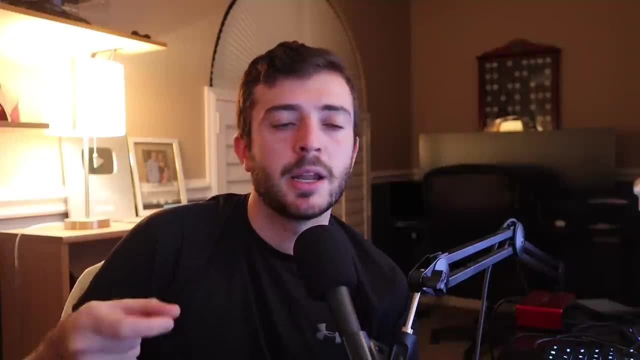 expectations when you are approaching an entry-level job in security. Do not underestimate your value. So I'm not saying you should negotiate for, of course, a lower salary, but set a realistic expectation. Saying all of this, unlike many positions out there, 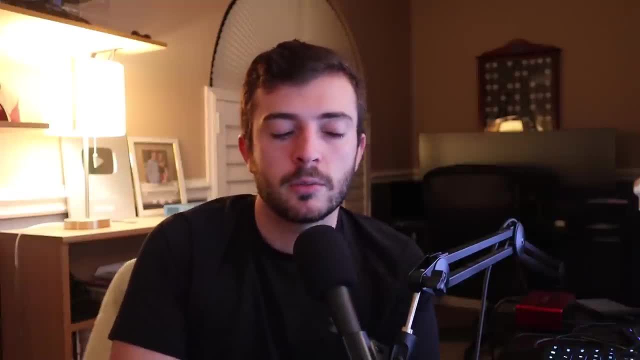 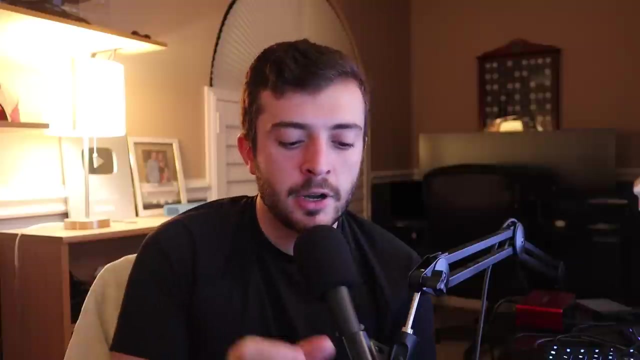 a cybersecurity career definitely will fast-track or put you on a track to earning a high-level. if you play your cards right, you work your way up. you have qualifications, of course, a lot of the different factors, But starting out with zero years experience, you probably shouldn't expect a super high salary Overall with numbers. be realistic Sometimes the higher the salary, the more time and responsibility you have for the job. Choose whatever balance you want. And this leads me into my next point, which is just the level of general. 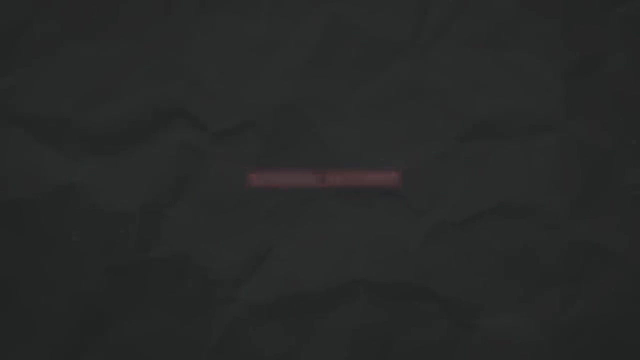 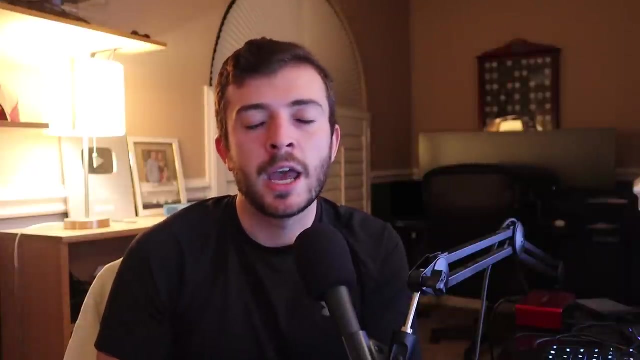 interest within IT technology and security. Measuring your level of interest and overall commitment to the topic of IT security or cybersecurity can help you be more successful and just more satisfied with your job. Anyone can be successful in this industry If you have. 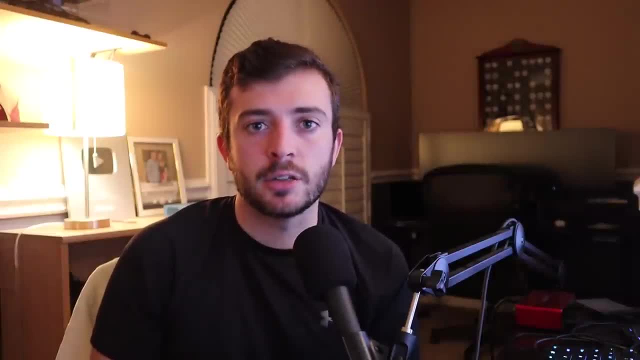 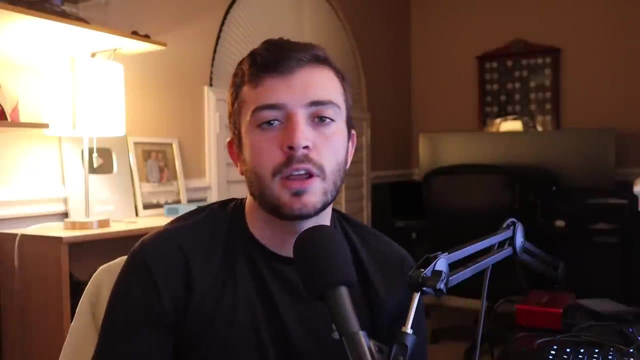 the drive, the commitment, the ambition you can accomplish and learn in this industry. It's great that you can learn basically everything online for free if you wanted to. So having a certain level of interest and general curiosity towards security is going to help push you during the 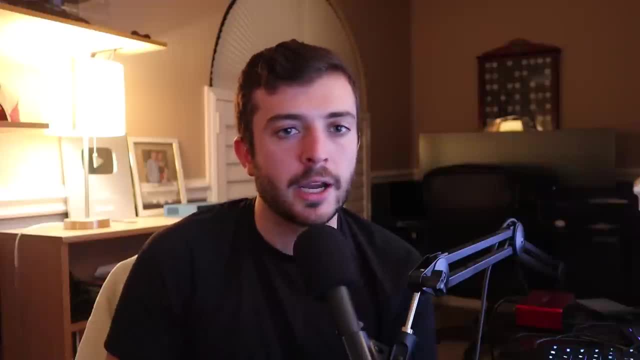 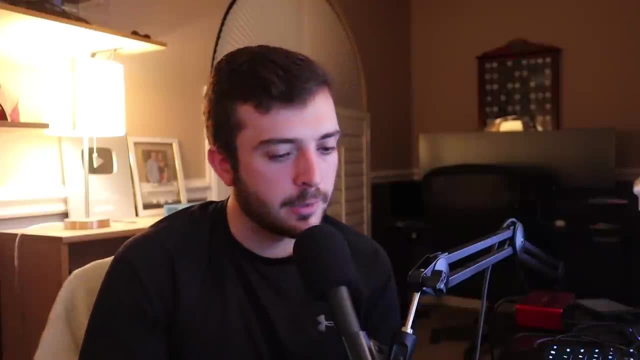 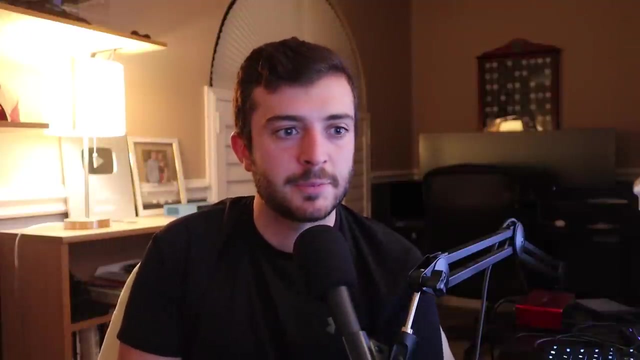 times where you perhaps may not feel like learning or doing something, And like any career in technology, the industry is, of course, ever-evolving, meaning you're always going to have to be learning something new and getting ahead, because this industry never stops. So 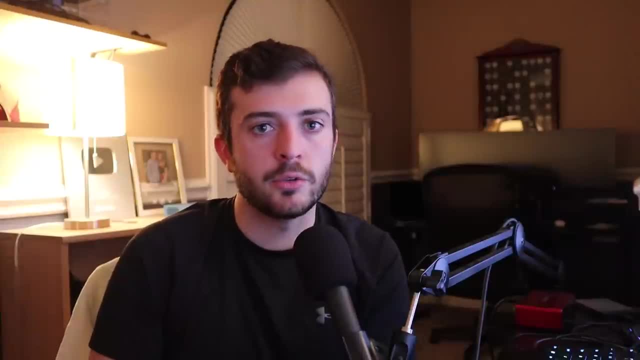 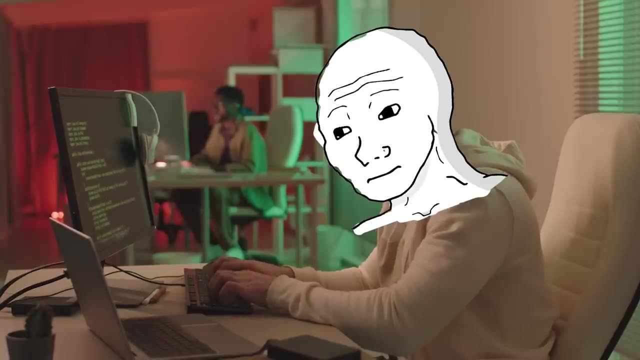 having some level of interest and pride in the work you do can help push you forward During those tough times. if you're chasing the high income insecurity but you're completely miserable while you're doing it, I mean, what quality of life is that? I mean that's up to.